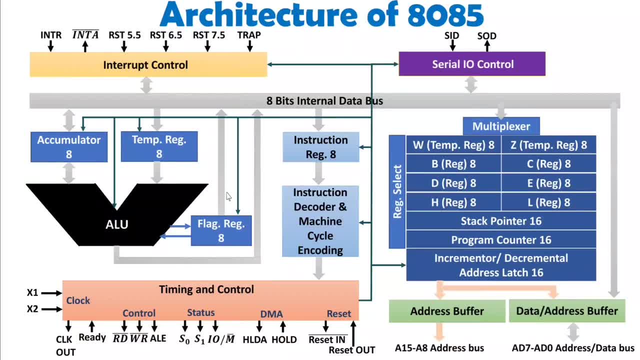 8085.. Here we are having arithmetic and logic unit that is performing arithmetic operation. Here we are having interrupt control that is to perform interrupt and service routine. Here we are having serial IO control where we want to have serial communication. So for that. 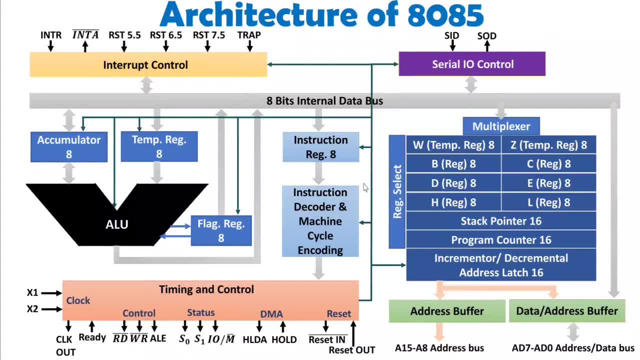 serial in data and serial out data is there, And here instruction resistor and instruction decoder segment is there, Right? So that is how complete architecture is there. But let us try to understand this architecture step by step so it will be more clear and you can easily remember how this. 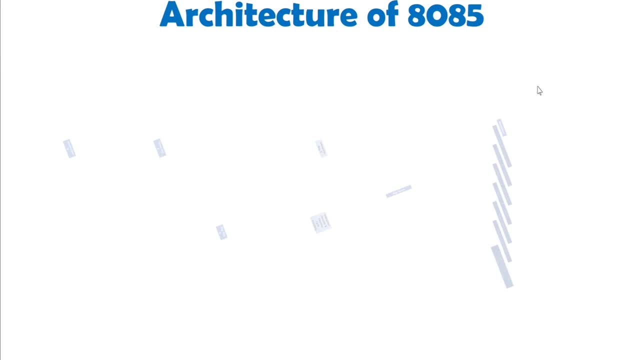 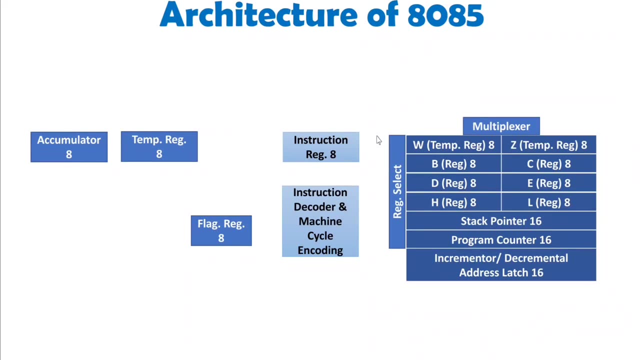 architecture is getting formed. So, my dear students, first of all you should know how many resistors are there with 8085.. So this section that explains you programming model of 8085.. And in this programming model we are having seven general purpose resistors. You see this. 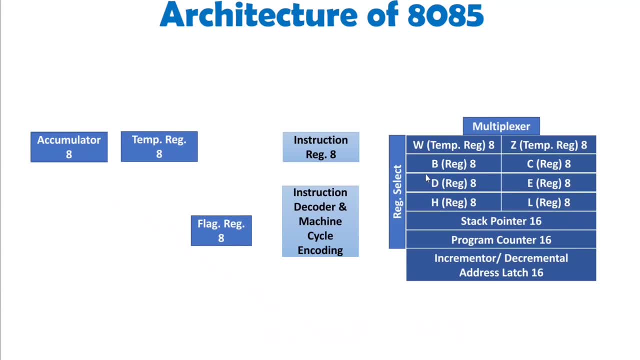 one resistor, that is accumulator, and then B, C, D, E, H, L. So these resistors are general purpose resistor. Why it is referred as general purpose resistor? The reason is programmer can do programming by using these seven resistors, And here I have written eight. What it means: 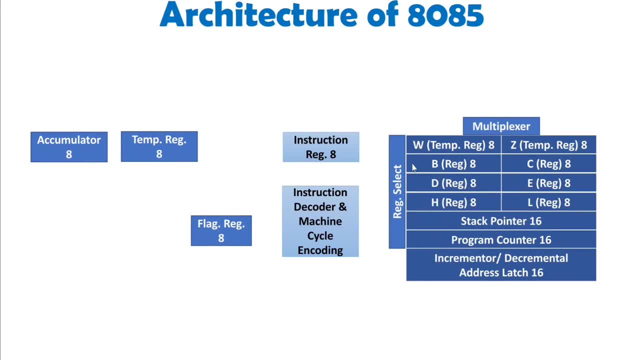 These resistors are having size of eight bits And these are general purpose resistors. After that, you see here we have stack pointer. This stack pointer is indicating top of stack and its size is of 16 bits. After that, you see here we have program counter, So that is also of 16 bits. 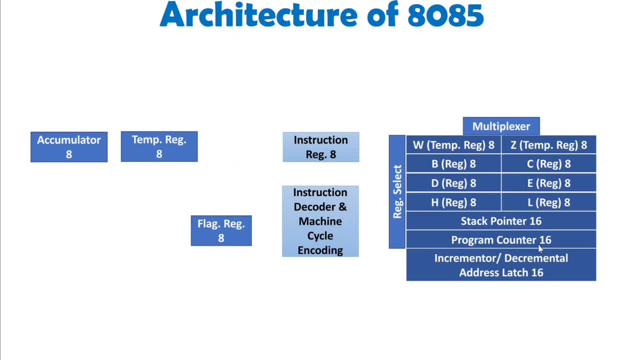 It is indicating where our next instruction is there in the memory Right. So next instruction location will be addressed by this program counter And after that incrementer and decrementer is there This incrementer operation. that is happening with program counter. Once one instruction is getting executed, program counter will get incremented by. 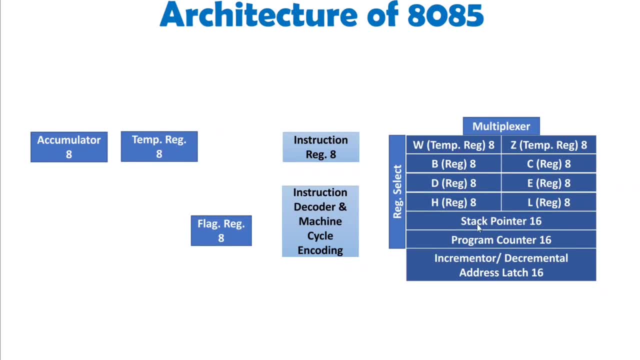 one automatically. For that. there is incrementer For stack pointer. there can be incrementer and decrementer operation For stack operation. I will be making separate video in which I will explain you how push and pop is happening and how stack is operated with 8085.. Here, just understand this stack pointer is used. 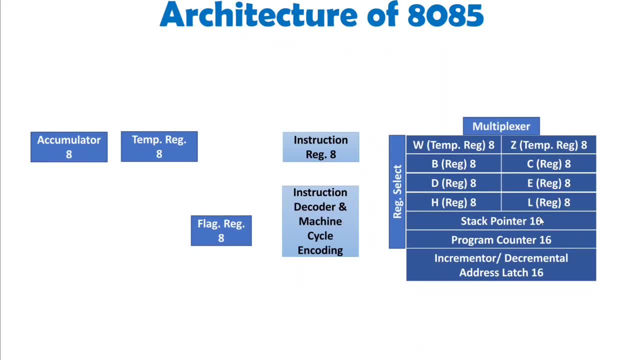 with stack operation in which push and pop that we do it with 8085.. And with push we will be having decremental of this address. latch So it will decrement stack pointer. pop will be incrementing stack pointer After execution of each instruction program counter. 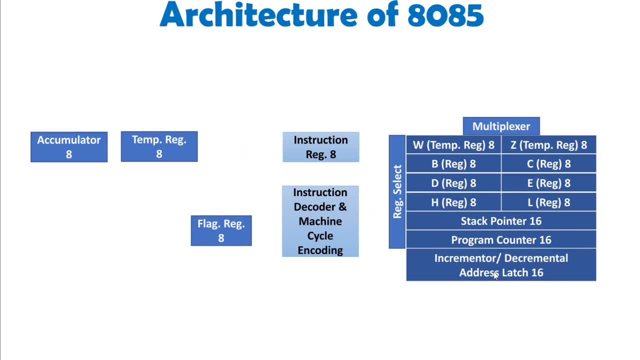 will get incremented by this incremental address. latch Now here you might be thinking what is happening with this WNZ? These are a temporary register and these are not available with programmers and these registers are used by 8085.. So internally there are some functions, which is: 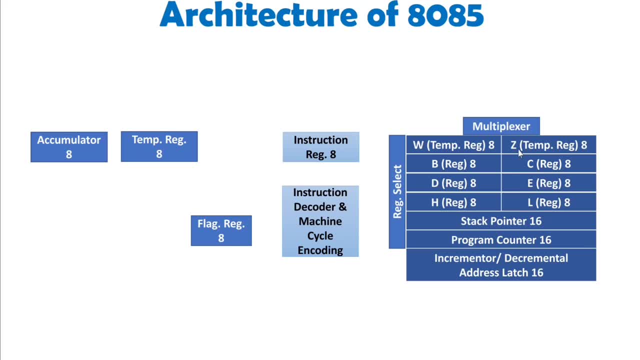 happening with WNZ. For some instructions, I will be separately explaining you how WNZ is utilized by 8085, but this is not available for programmer. Now, my dear students here, temporary register is there, as well, as flag register is there, So that we will discuss once we have ALU. 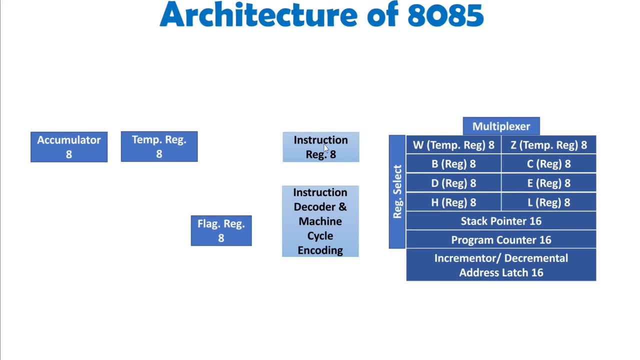 operation and here we have instruction register and instruction decoder. That you understand. I will explain you when I explain how this 8085 is functioning. In this video only we will be learning that Let us see first how internal structure is there. So you see here this: 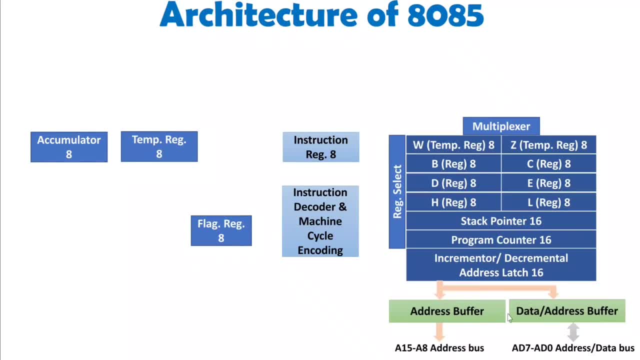 programming model that is connected with address and data buffer. There are total 16 address lines A0 to A15 and total 8 data lines D0 to D7. But you observe here AD0 to AD7, AD2 to AD8 and AD3 that are connected with address and data. So it is the same function That is. 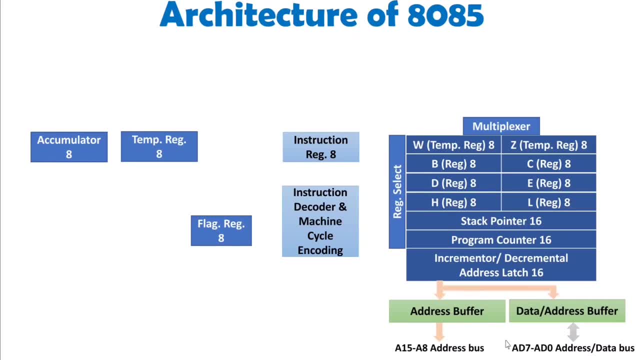 how address data lines are time multiplexed, So on same line there will be address as well as data and that we need to separate by using address latch. enable that. we will discuss it in some other video. But remember one thing: with 8085, we have total 16 address lines and 8 data lines. Now this: 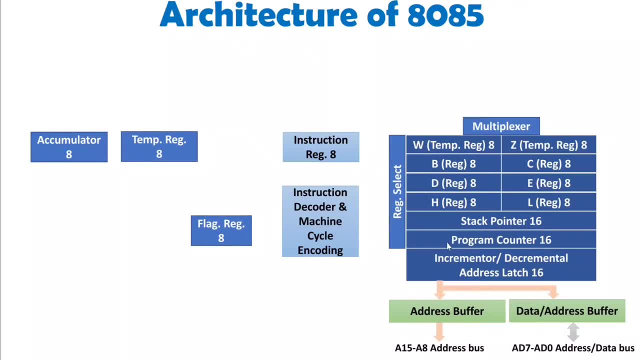 that will be indicated by program counter right and whatever address is there, that address will be there with memory and from memory we will be executing instruction for that. i'll give you one complete example so that will be more clear. first you just see how architecture is there. 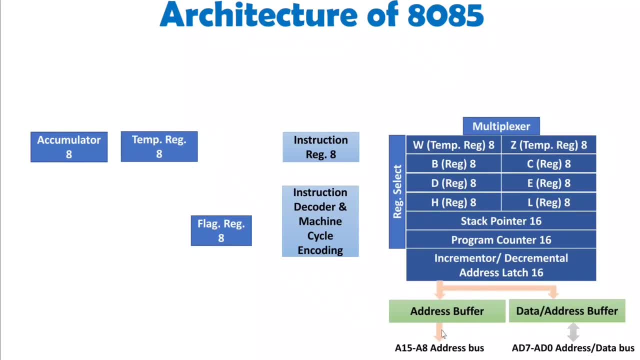 so, my dear students, once you understand these are the address lines and data line, you need to understand internal data bus. so, whatever data that we fetch it from here, that data bus is connected internally. so you see, i have shown it over here and after that, here you see timing and 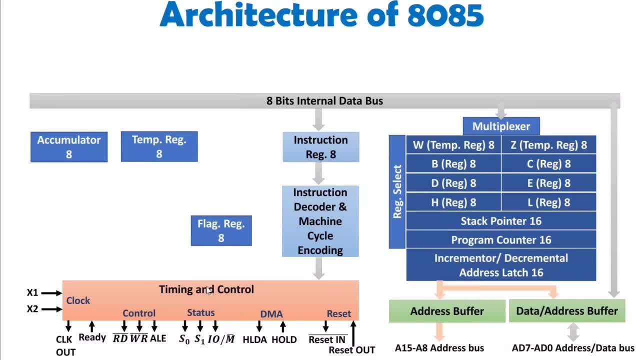 control unit that is been connected over here, and once you understand timing and control unit, you will be able to understand how alu is connected over here. i'll be discussing everything in detail, so don't worry about it. now. you, if you observe this timing and control unit and arithmetic and logic unit, so that is connected. 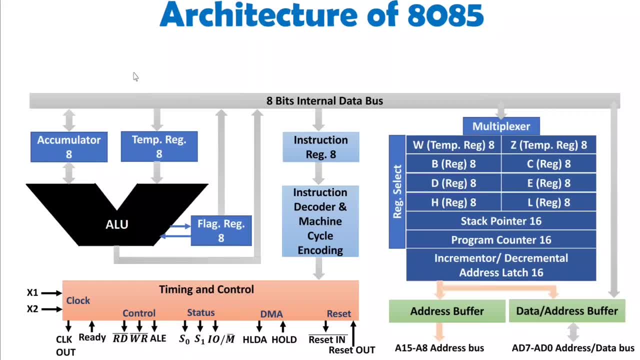 over here, as you can see it in this figure, and here we have interrupt control segment, in which we have intr, inta and rst 5.5, 6.5, 7.5 and trap interrupt signal. and over here you see, we have serial io control, in which serial input data and serial output data is. 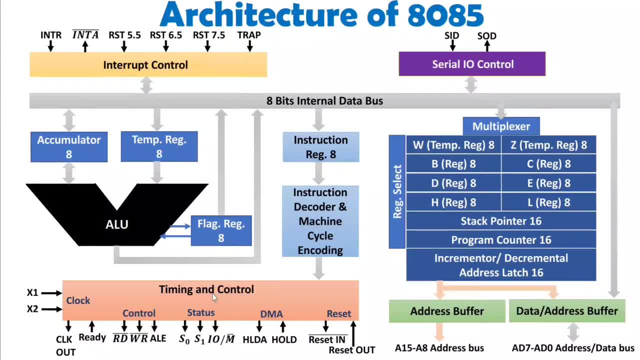 there and this timing and control unit that provides timing and control to enter microprocessor 8085. you see, it is providing timing and control to enter microprocessor. right now, let us try to understand how this entire architecture is functioning by one practical example. so, my dear students, first of all you should understand: microprocessor 8085 does not have its own memory. 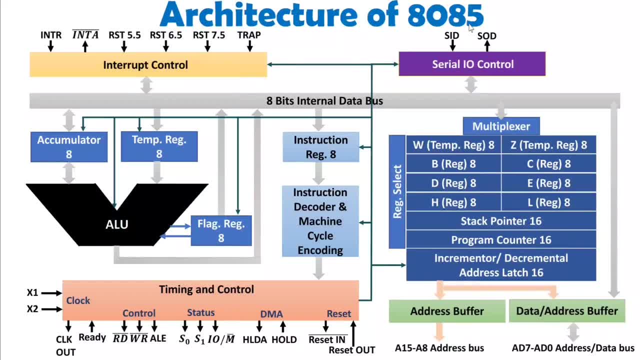 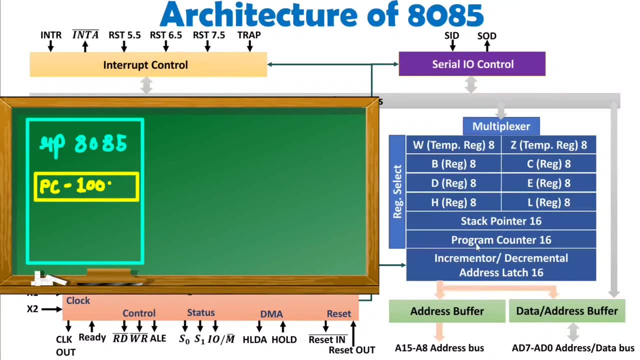 so we actually need to understand how this entire architecture is functioning by one practical example. to understand how this entire architecture is functioning by one practical example: externally, interface 8085 with external memory. now that external memory will be having address and data right, this external memory will be having address and data. now, here program counter will be. 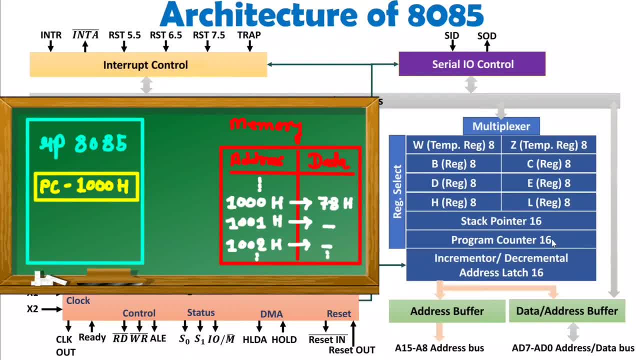 indicating address of next instruction. so once we give signal to 8085 that execute program, then what will happen? it will be having address of first instruction in program counter. So what it does is it will be giving signal to memory and at that particular address, whatever data is there that it will. took it from AD0 to. 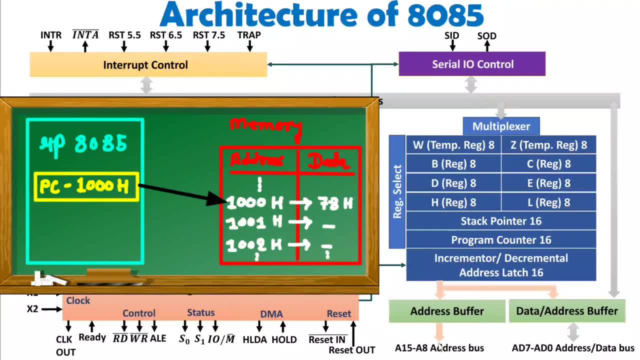 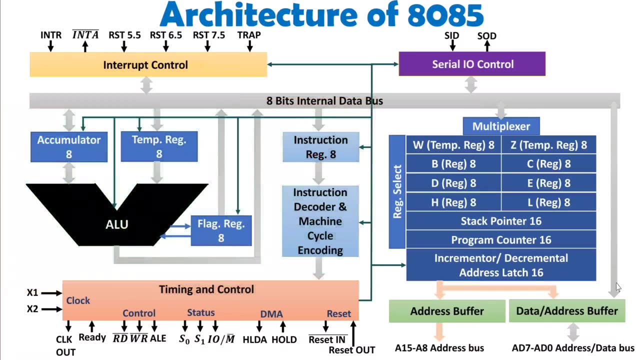 AD line. So first it will give address to memory. Once it give address to memory it will read that data which was there on that memory. and those data- those are D0 to D7- that will get fetch inside. If you see my previous video, in that I have already told you microprocessor 8085. 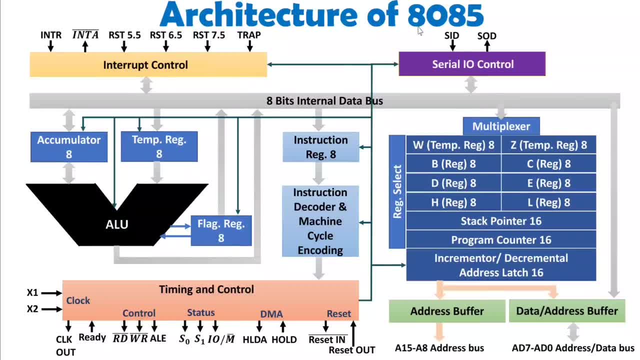 executes instruction in three steps: First is fetch, second is decode and third is execute. So first step is what? First step is fetch. Fetch means what? First of all, program counter will indicate address from that address of memory. it will fetch the data Once that. 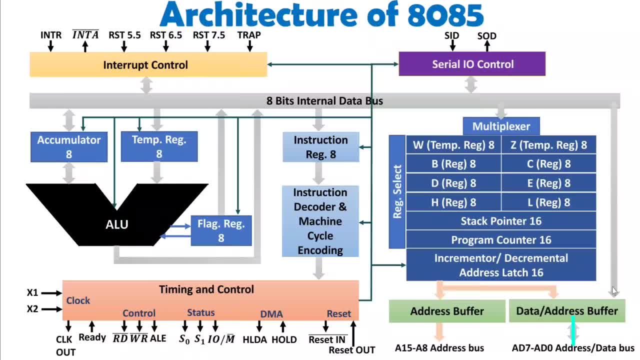 data is fetched, it will give address to memory. So first step is fetch. So first step is fetch. That data that will come inside means it is getting fetched. Once that data is getting fetched, that data will go in instruction register. Once that data goes in instruction register, it needs. 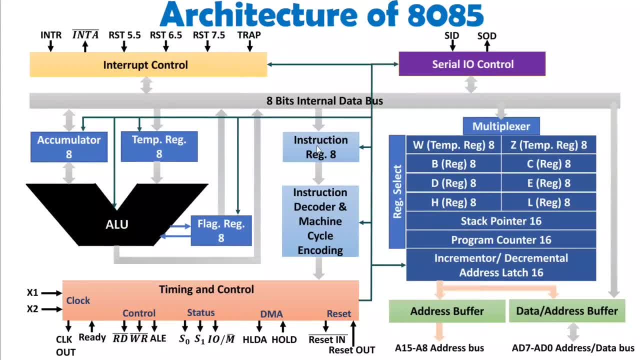 to identify that, what operation should be getting done, and based on that, this data that will go in instruction decoder. So now second operation will get start, that is, decode. Decode means what Microprocessor does not have idea what has to be done. Decode will tell you that what has to be. 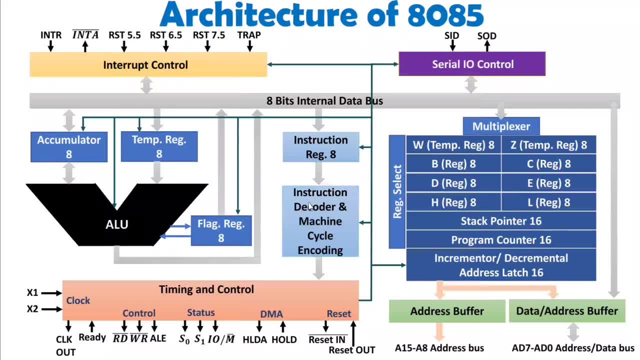 done So. in second stage there is a decode operation and in that decode operation this block will identify what operation has to be performed. Once it identifies what operation has to be performed, that will be given to timing and control. So timing and control will be having idea what 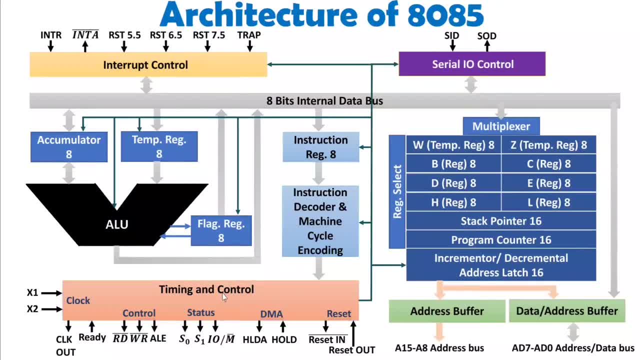 operation has to be performed. There can be multiple operation, There can be move operation, There can be add operation, There can be any operation as per instruction, Right. So once it is having that idea that what operation should be performed, timing and control, that will be giving. 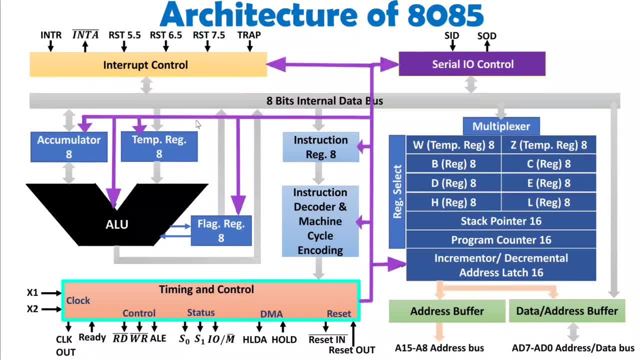 timing and control to each of the blocks which are there inside Right Now. let us take example, like here: program counter is indicating one address and in that address there is operation which is add B Right. So for add B, whatever opcode is there that is coming. 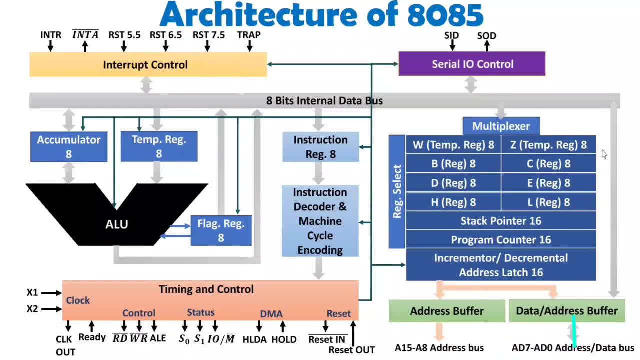 inside over here on data bus, So that opcode will come over here first at instruction register. That instruction register will take that opcode and that it gives to instruction decoder. So that will be second stage in which instruction decoder will identify what operation should be done. 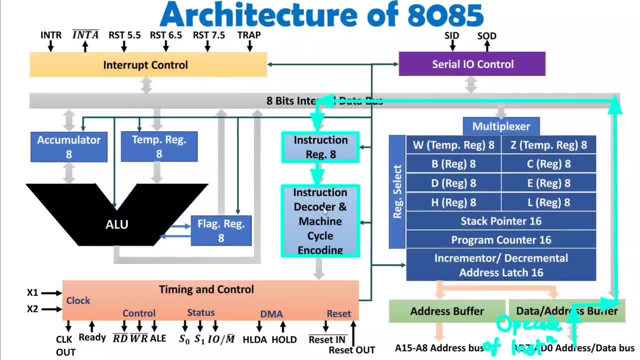 Now here add operation should be done. So for add operation it needs to give timing and control to this block, and once execution is getting initiated, timing and control will tell ALU that you will have to perform add operation. So with ALU, here there are two resistors, you see. 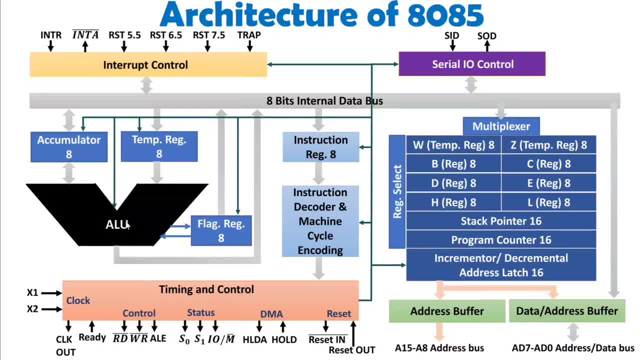 Here these two resistors are operand of this ALU. that you can say, And with A architecture of 8085 you can say: this accumulator is fixed operand, So one operand is fixed. Second operand, that could be B, C, D, E, H, L, it could be any other resistor, But one operand is fixed. Now, here I want to. 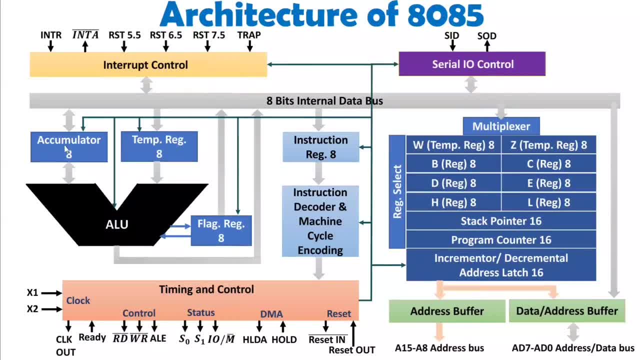 execute add B. So add B means what One operand is accumulator. Second operand is B. Both will get added and once both are getting added, output will come over here. that will get stored in accumulator again And, with respect to operation, flags will get changed. Flags will show. 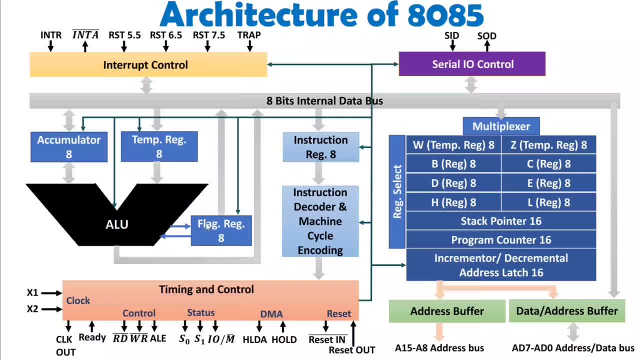 you. status of the 8085.. So flag resistor is 8 bit resistor, in that S, Z, A, C, P, C, Y. S stands for sign, Z stands for zero, A, C stands for operation, Z stands for operation. Z stands for operation. 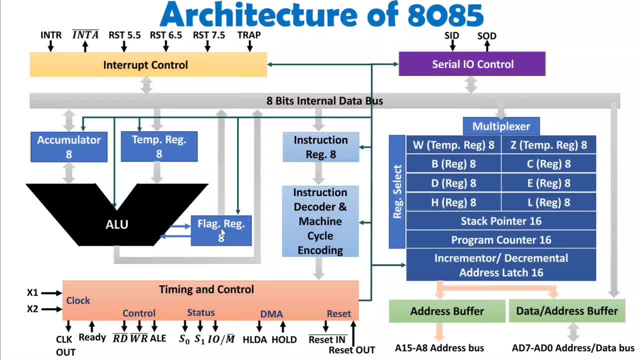 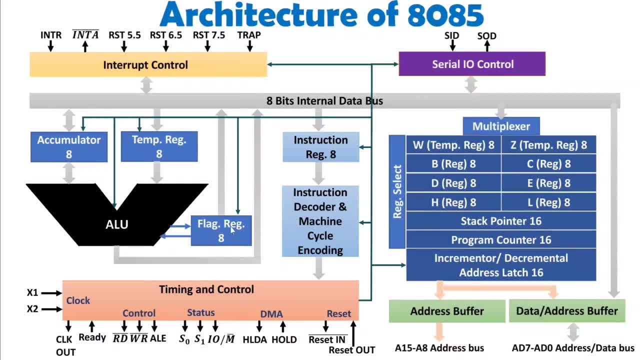 observing after every instruction. this flag resistor is getting modified by ALU and it is bidirectional UC. The reason is: ALU needs to be modified, So ALU needs to be modified. So ALU needs to be modified, So ALU needs flag resistor as well as whatever operands are over here. So, along with 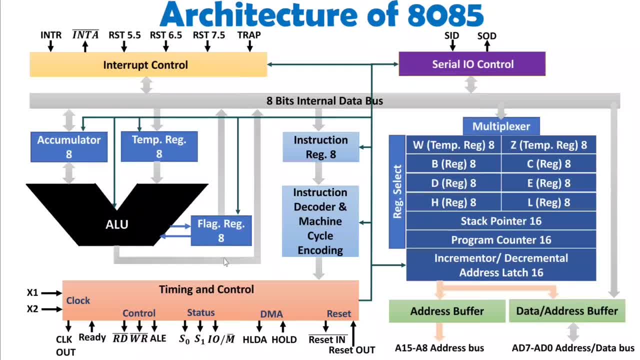 operands and flag resistor, it will perform complete execution and it will give output, This interrupt control, that is, having interrupt service routine, and there are many things. for that I have made separate video for this And this serial communication that even I will be explaining you separately. So right now you just consider that in this way. 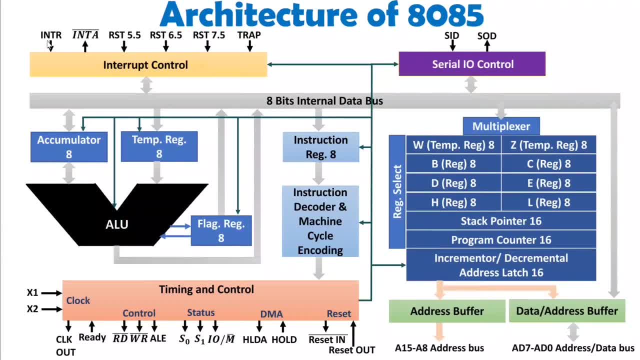 Interrupt control is having INTR interrupt request, INTA bar interrupt acknowledgement line. And then there are 4 hardware interrupt: RST 5.5, 6.5, 7.5 and trap Trap is non-maskable interrupt. And here 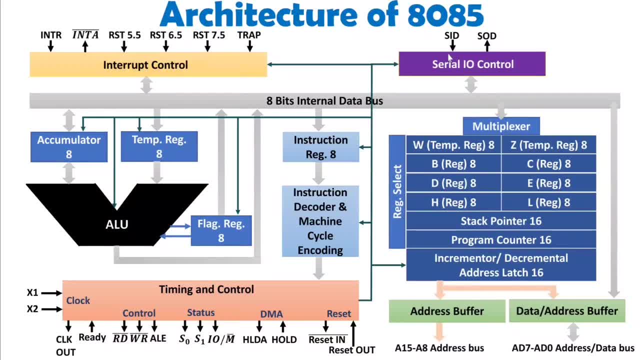 SID and SOD. those are 2 lines which is there for serial communication, So serial IO control is there. So, my dear students, whenever you want to execute any program, it will happen in step by step execution, So it will execute one instruction In single instruction. 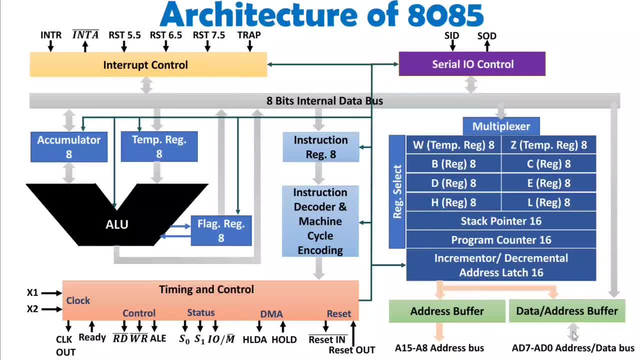 execution. there are 3 stage. At first stage it will fetch instruction. For fetch instruction over this AD0 to AD7 line. it will be taking data and that data will go inside. It will go inside this instruction resistor. In second stage there will be decode operation. In decode operation, this: